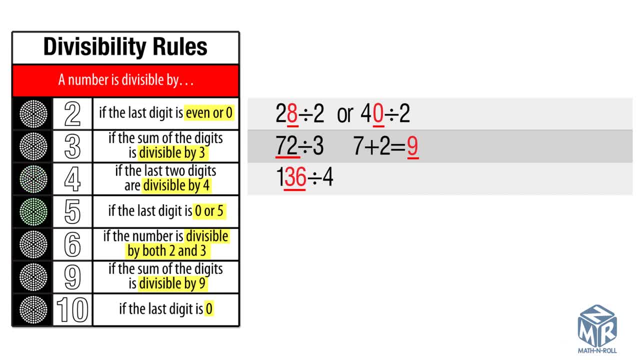 by 4.. A number is divisible by 5 if the last digit is 0 or 5.. 60 divided by 5.. The last digit is 0,, so 60 is divisible by 5.. 75 divided by 5. The last digit is 0,, so 60 is divisible. 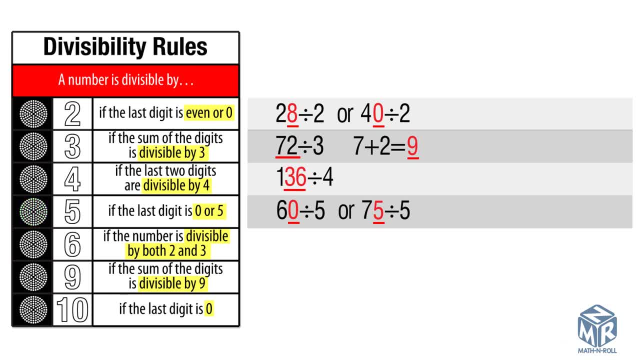 by 5, so 75 is divisible by 5.. A number is divisible by 6 if the last number is divisible by both 2 and 3.. 18 divided by 6.. 18 is divisible by both 2 and 3, so 18 is divisible by 6.. 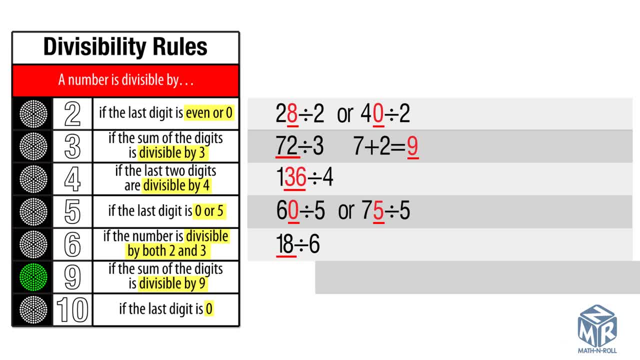 A number is divisible by 9 if the sum of the digits is divisible by 9.. 198 divided by 9.. 1 plus 9 plus 9.. 1 plus 8 equals 18.. 18 is divisible by 9,, so 198 is divisible by 9.. A number is divisible. 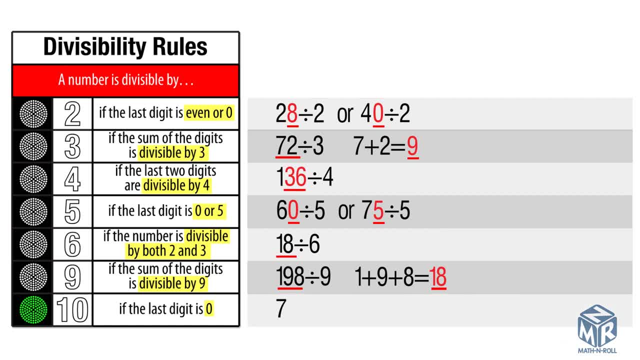 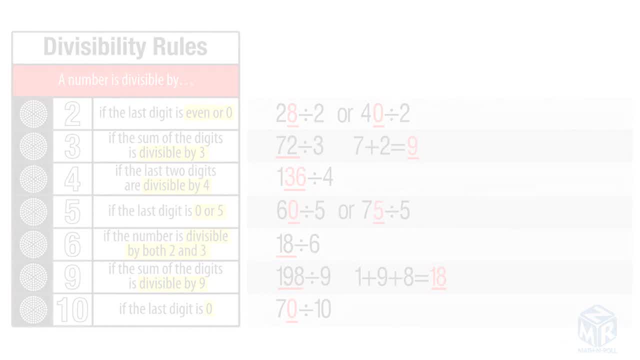 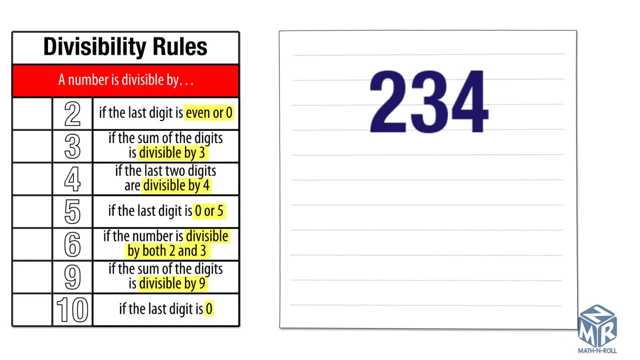 by 10, if the last digit is 0.. 70 divided by 10.. The last digit is 0,. so 70 is divisible by 10.. Let's look at 234 and figure out which numbers it is divisible by. Let's check if it's divisible. 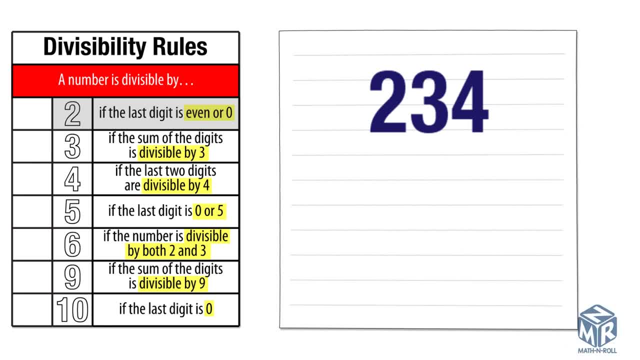 by 2.. The last number is even, so it is divisible by 2.. Let's check if it's divisible by 3.. The sum of the digits is 9, and 9 is divisible by 3,, so 234 is divisible by 3.. Let's check. 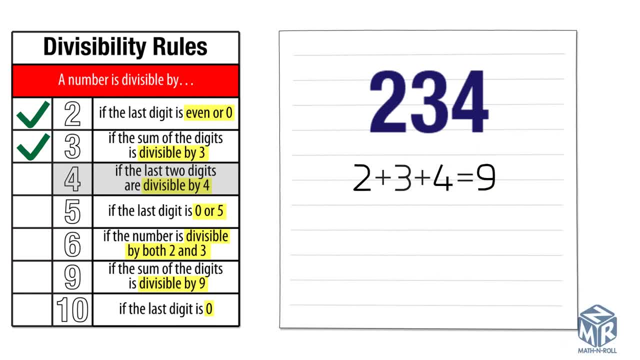 if it's divisible by 4.. The last two digits are 34,, and 34 is not divisible by 4, without a remainder. so 234 is not divisible by 4.. Let's check if it's divisible by 4.. Let's. 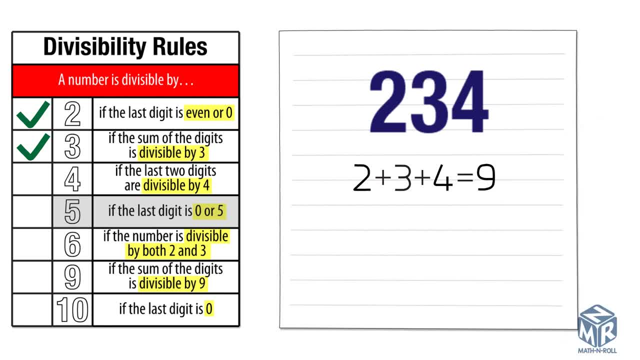 check if it's divisible by 5.. Let's check if it's divisible by 5.. The last digit is not 0 or 5, so it is not divisible by 5, without a remainder, Let's check if it's divisible by 6.. 234 is divisible by both 2 and 3, so it is divisible. 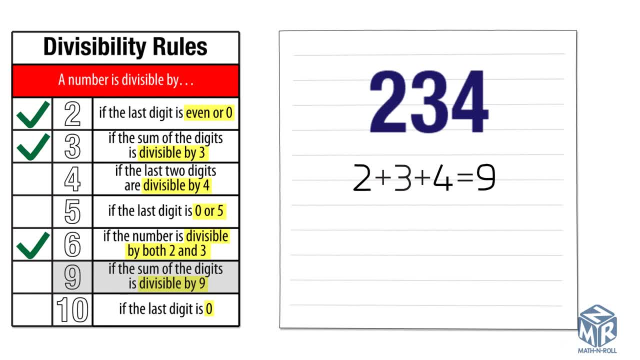 by 6.. Let's check if it's divisible by 9.. The sum of the digits is 9, which is divisible by 9, so 234 is divisible by 9.. It is not divisible by 10 because the last digit is not 0.. Using the divisibility rules, we see: